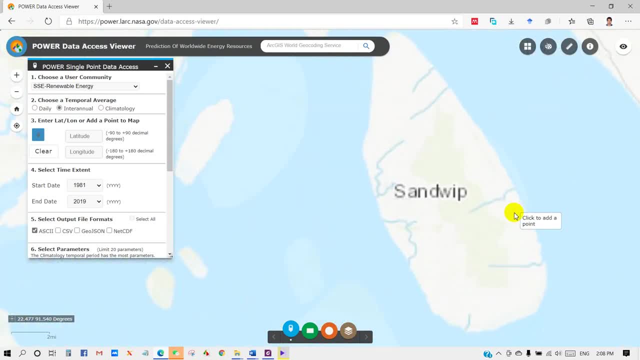 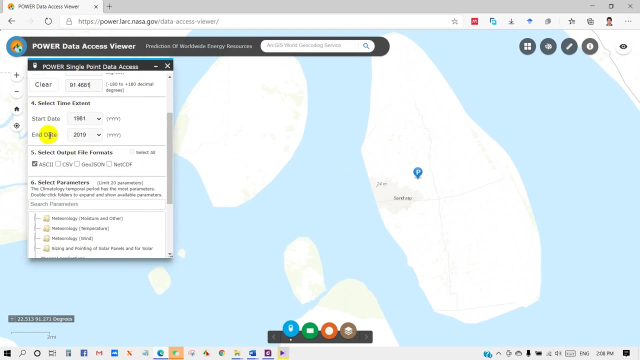 As my location. After that, you will get the latitude and longitude of this area. Now I will select the time extent. Here I am selecting it from 1981 to 2019.. so here you have to choose the output file format. here there are several. 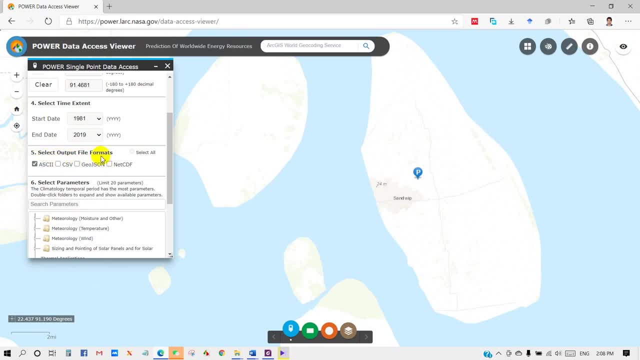 formats, but I am choosing CSV to get the file in Excel from here. you can also select the parameters. here I am selecting those data that I need. you can select or choose your your data according to your need. here I am just selecting precipitation, relative humidity, and like this I am selecting my 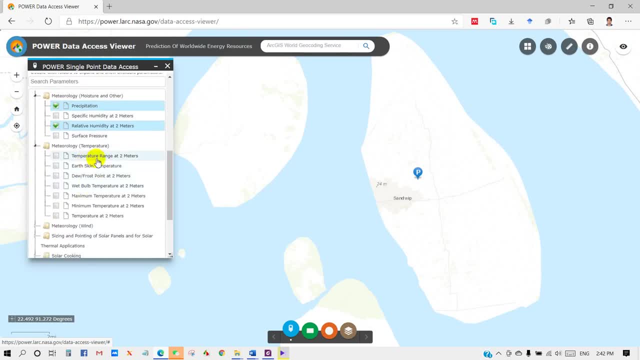 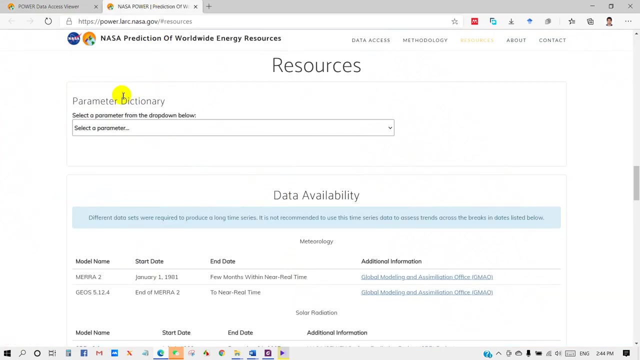 other design data. here I am selecting precipitation, relative humidity, and like this I am selecting my other design data data. if you really want to know what does the parameter means, then just click on the parameter definition here. you will get a parameter dictionary from here. just select any parameter. 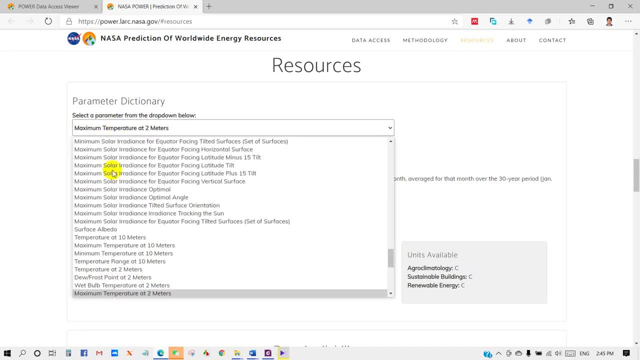 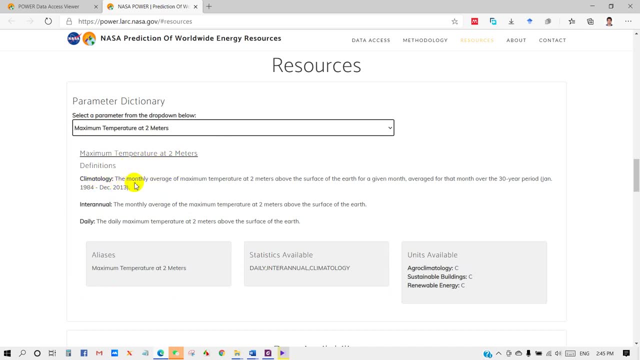 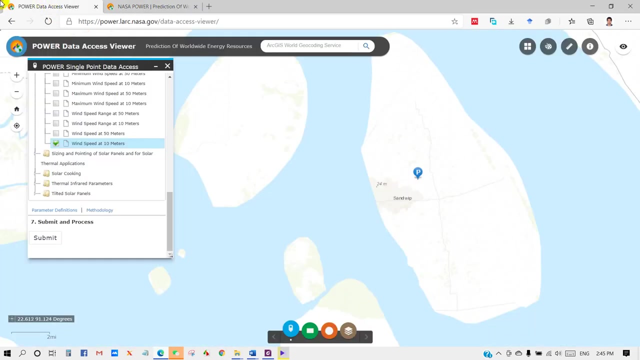 here. I have selected maximum temperature at 2 meters and all the definition comes. you can see from here what does it actually means in climatology, or interannual or daily? parameter dictionary is really very helpful to understand all the parameters properly. you can check this out. I'm going back to power access data viewer and checking all the options. 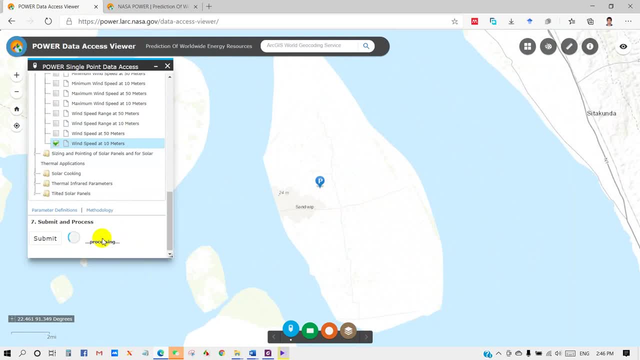 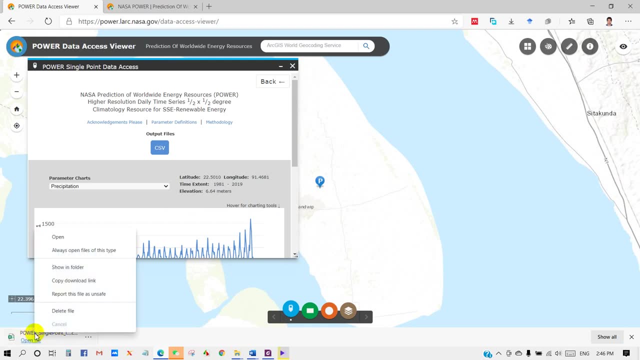 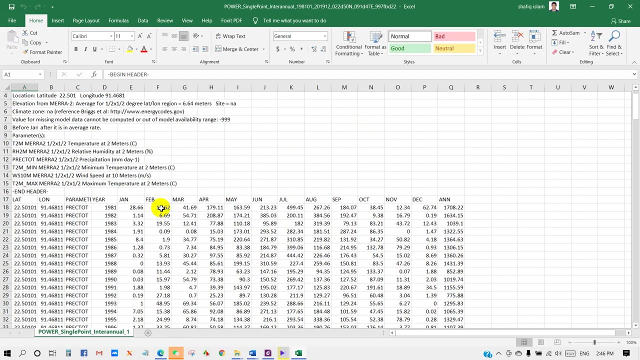 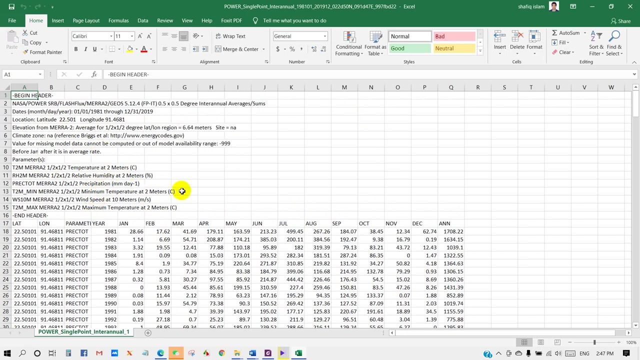 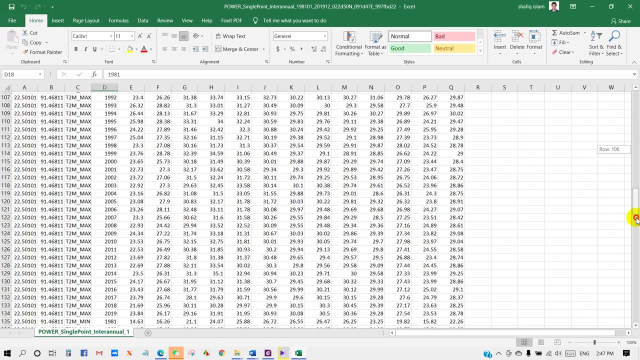 I'll just click on submit here. I got the output file. I'm downloading this CSV. just open your excel file here. you can see all the data has been downloaded here. I am just checking all the downloaded data. I got it from 1981 to 2019, as I have selected. 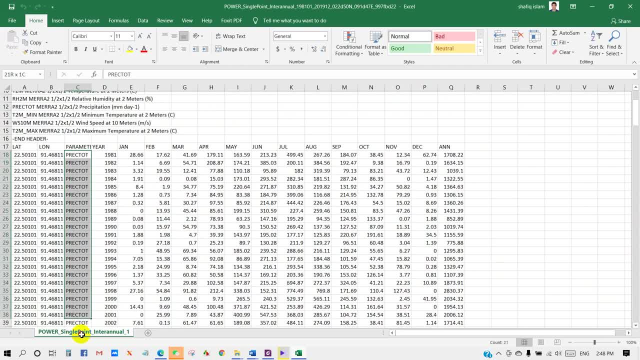 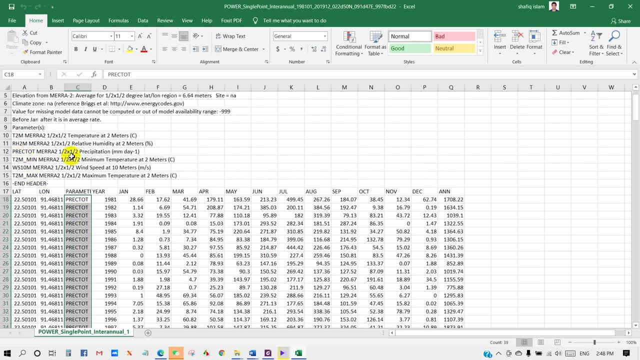 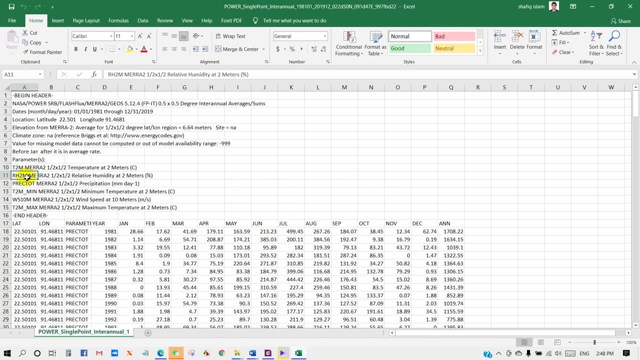 all the data I downloaded. and here I'm just going to open my browser again. now I'm actually going to open the library window and I'm just going to wait it to load and I'll click here and it will ask me to load all the data. so I'll just 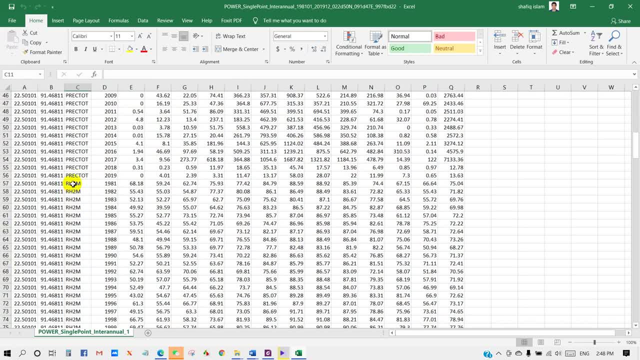 click on here and it'll tell me where all the data has been downloaded. it already has been downloaded. I can also open my browser again and there it says the data has been downloaded here. I'll click on it and then it will ask me to load my data.